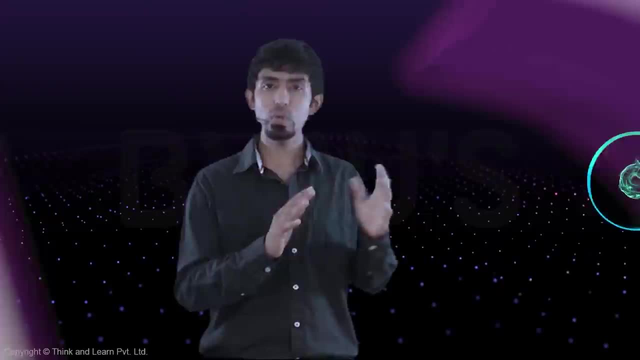 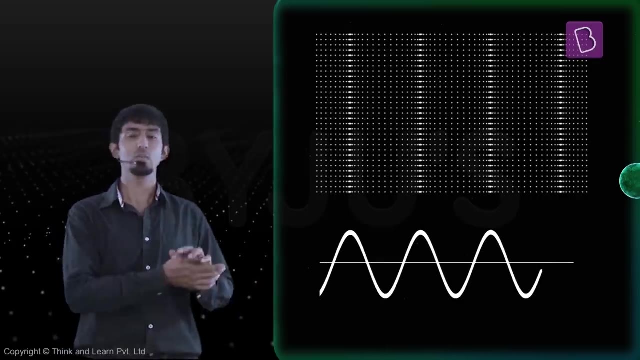 So we know that sound is a set of compressions and rarefactions, as you can see, and a better way to represent that is as waves in this format where you can see each compression as a peak and each rarefaction as a trough. So we're going to take that wave, keep it in front of us. 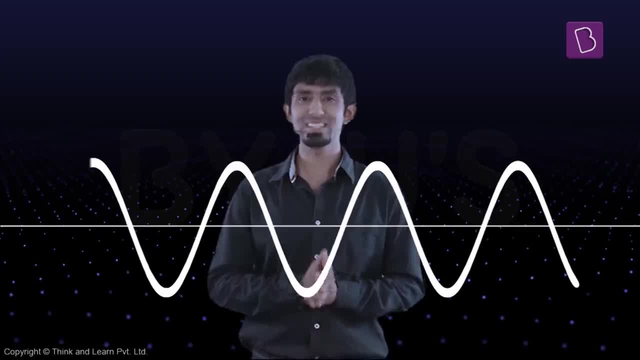 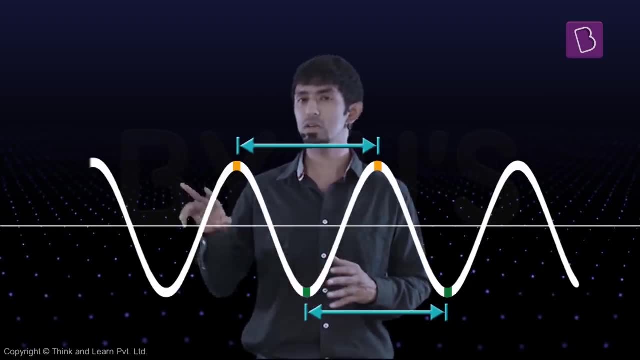 and we're going to define certain quantities, The first one being the distance between two crests or two troughs. You already know they're going to be equal. right, The distance between two crests and two troughs is going to be equal, and that particular distance is what 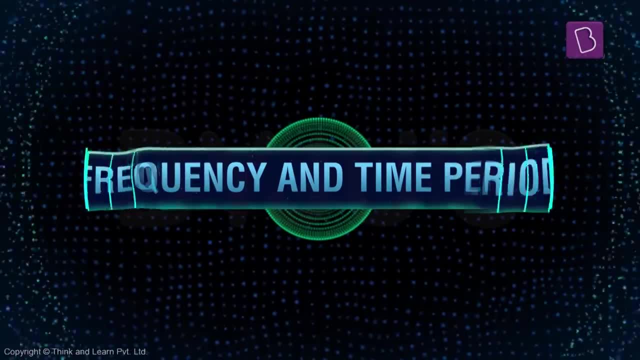 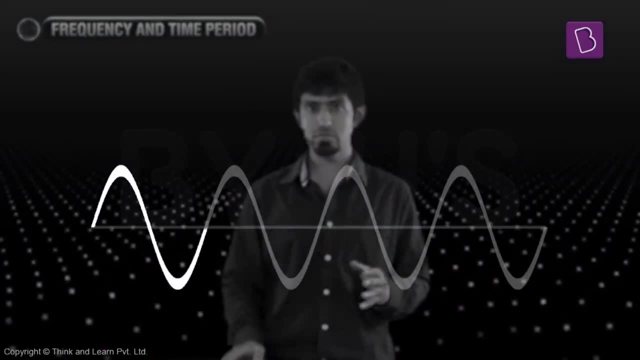 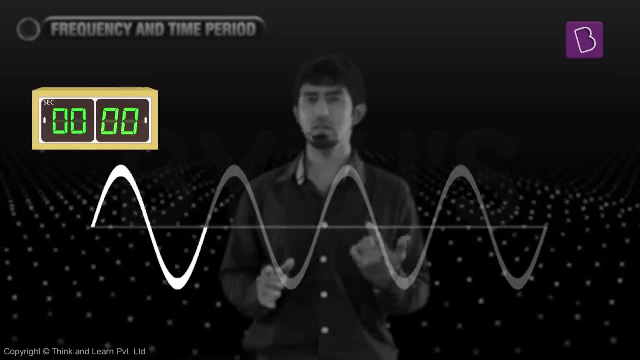 we're going to call a wavelength, So it's the length of this wave. Another thing we're going to define is how many such crest trough pairs. We take one crest and a trough. That's like one wave, because after that that keeps repeating, So that one crest and one trough in one second. 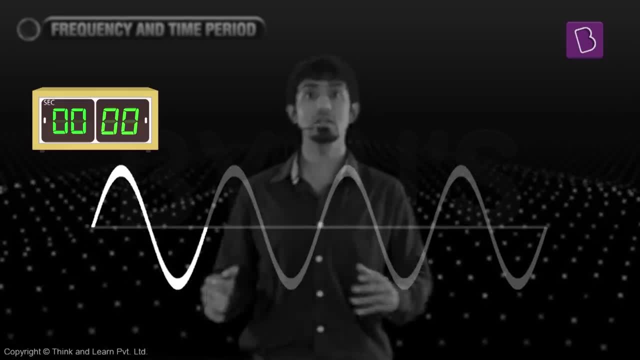 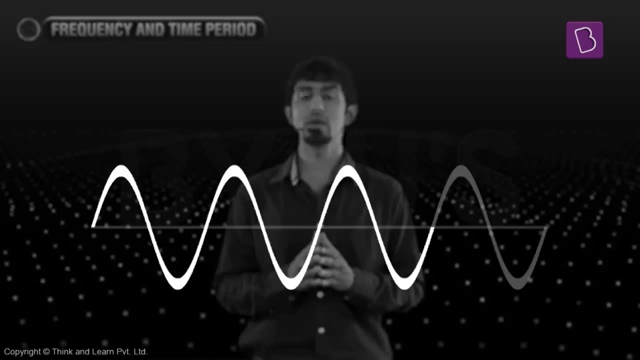 or in one unit of time, usually it's a second. How many times does it occur? So if you have three of them occurring right In a second right- One, two, Three- Then you have a frequency of three. If you have four, it's four and it's beginning to get. 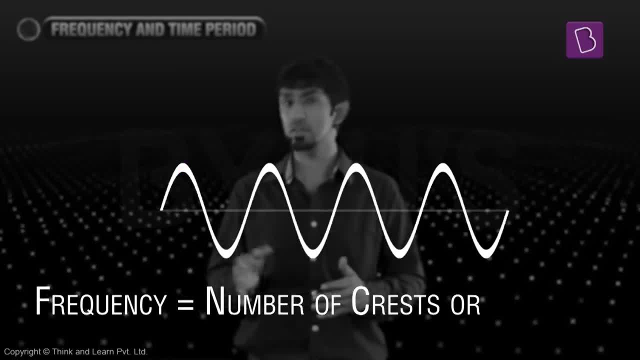 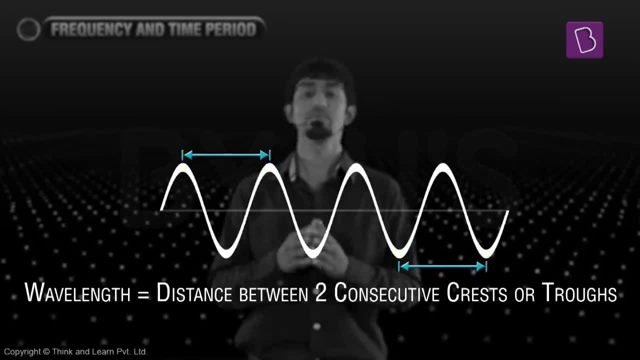 obvious now, isn't it? So your frequency, which is the number of crests or troughs in a unit of time- usually a second- And wavelength is the distance between two crests or two troughs. And now you have to calculate something called time period. right Now, it's very easy to calculate. 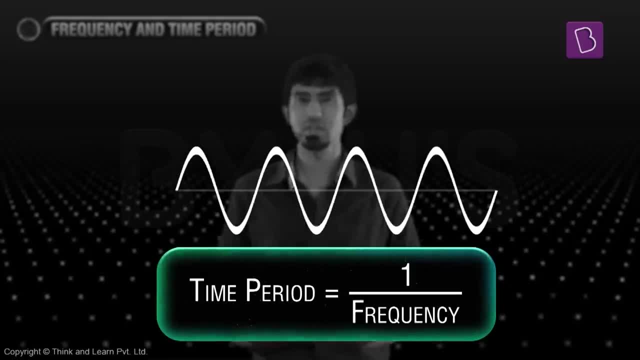 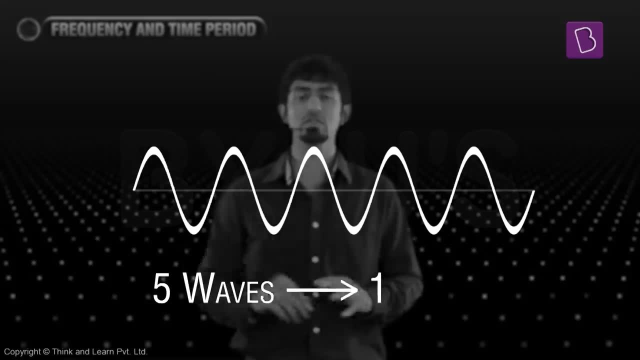 that that's going to be exactly one by the frequency. Now, why is that true? From now, let's just call it waves. okay, A crest and a trough put together, let's call it one wave. So therefore, let's say I have five waves in one unit of time, in one second. Then what is my? 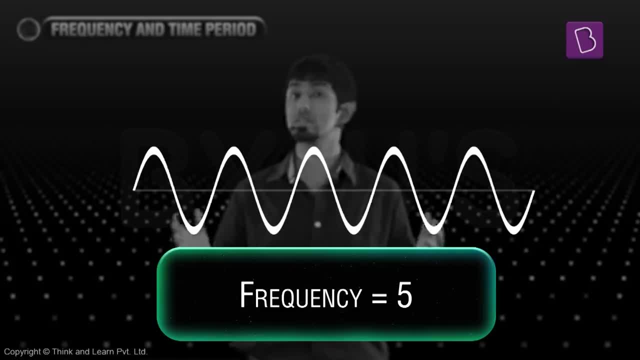 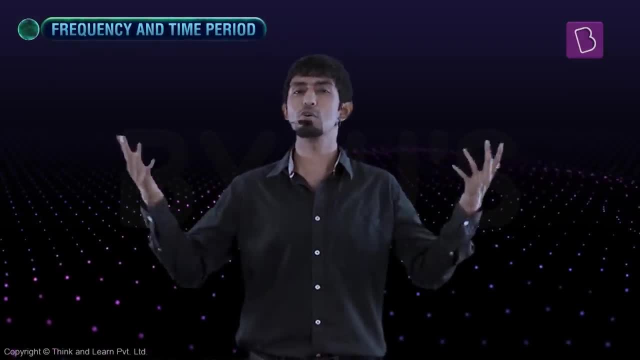 frequency? Yeah, five in one second. Therefore, the frequency is five. But now if I were to ask you what is the time period, In other words, how long does one wave take? This goes back to the old question, right? Five mangoes cost 20 rupees. How much does one mango cost you? Yeah, you would. 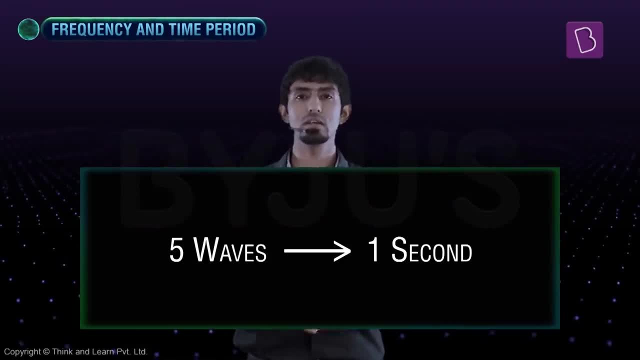 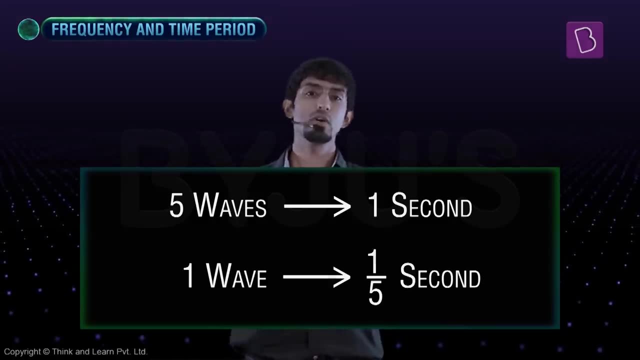 do this pretty easily, wouldn't you? If five waves take one second, then one wave will take one by fifth of a second right. That's exactly what it will take If 10 waves take one second and the frequency is 10, then how?